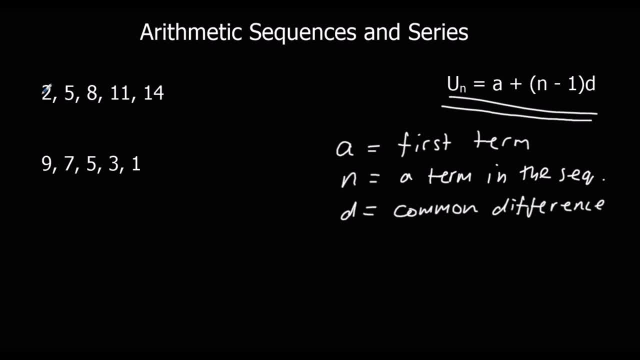 Okay, so looking at the first sequence over here, A would be two because it's the first term. A is two. And D, the common difference is three. So the first term is two and it goes up. And D goes up in threes. So for this sequence, UN is two plus N minus one times three. So if we substitute any value of N in, we can find out a term in the sequence. So if I wanted to find the tenth term, so we can write U10, this is a notation, the tenth term is two plus 10 minus one. So we can find out a term in the sequence. So if I wanted to find a number approximately around N, we could find the tenth information in the equation. You want to do something about it. Again the tiefschutzm le as I just told you really nicely. 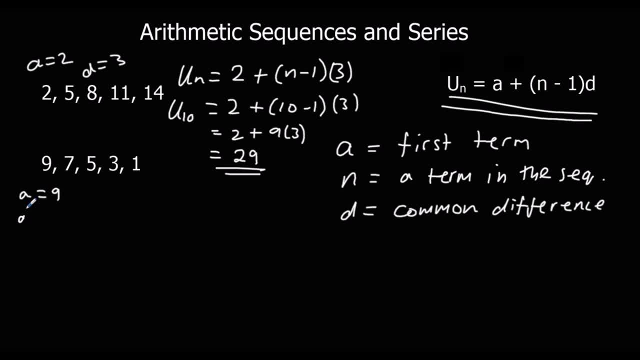 We're going to find a number. It's going to be 10 no more times eight. It must be three times nine. It's going to be 10 times nine, put that into this equation. And then we're going to do something about it too. You can imagine finding out this. 24 minus 11 plus one times three. Which is two plus nine times three, which is two plus 27, which is 29. So, 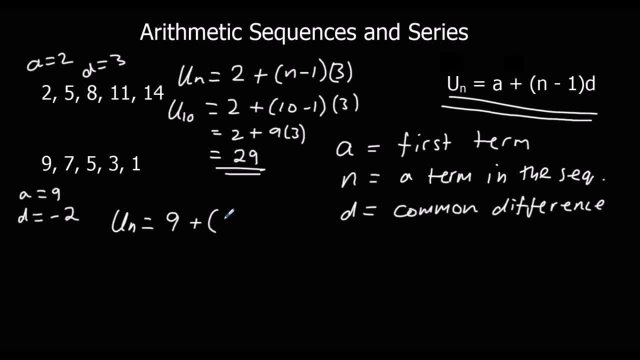 9 plus n minus 1 times minus 2. So again, if I wanted to find the 10th term of this sequence, which I'll call u10, the 10th term u10 is 9 plus 10 minus 1 times minus 2, which is 9 plus 9 lots of minus 2, which is 9 minus 18, which is minus 9. So the 10th term of 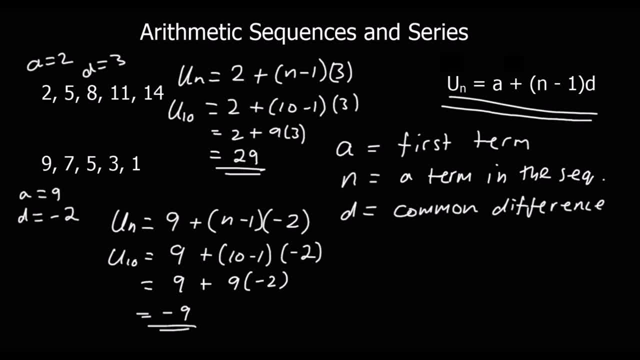 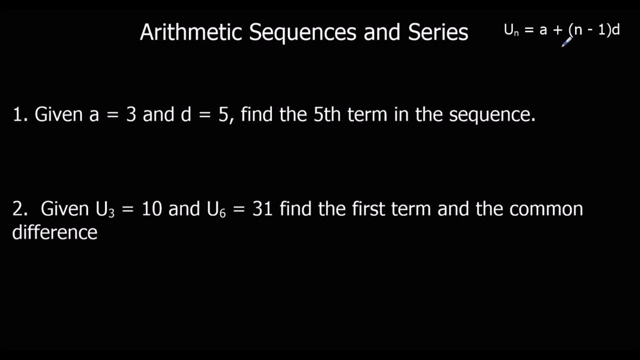 this second sequence is minus 9. OK, so we're going to practice using the formula. So we've got the formula up here. un is a plus n minus 1 times the difference. So a, the first term is 3, and it goes up in fives. What is the fifth term? 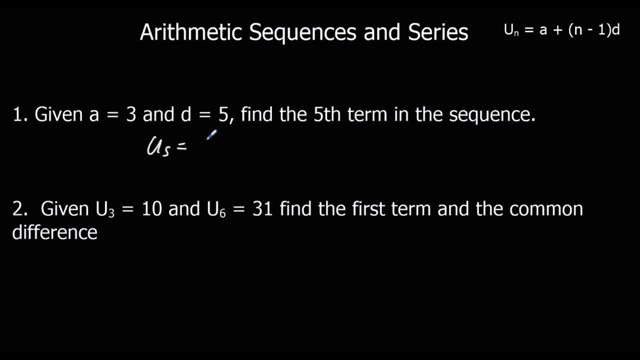 So u5, the fifth term, is a, 3, plus n minus 1. So we want the fifth term. So n is 5. 5 minus 1, lots of d, which is 5. So it's 3 plus 4 fives. 4 fives are 20, plus 3, 23. 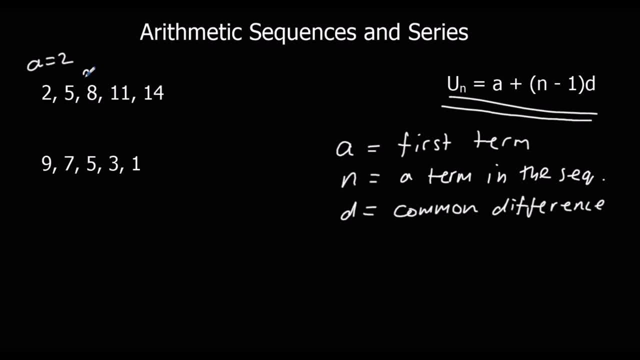 term A is two And D. the common difference is three. So the first term is two and it goes up And D goes up in threes. So for this sequence UN is two plus N minus one times three. So if we substitute any value of N in, we can find out a term in the sequence. So if I wanted 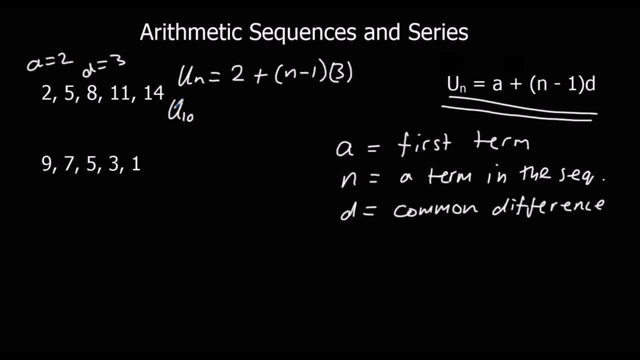 to find the tenth term, so we can write U10, this is a notation. the tenth term is two plus 10 minus one, So we can find out a term in the sequence. So if I wanted to find a term, we can this equation. So let's do. the term N comes up higher one times three. 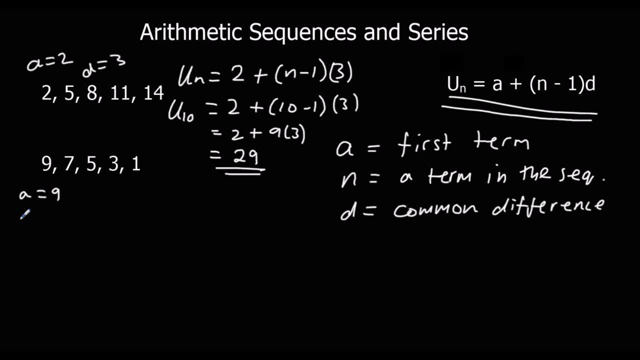 So we can use a vacation. we could choose two to the ninth. from each We could figure 9 plus n, minus 1 times minus 2.. So again, if I wanted to find the tenth term of this sequence, which I'll call u10,. 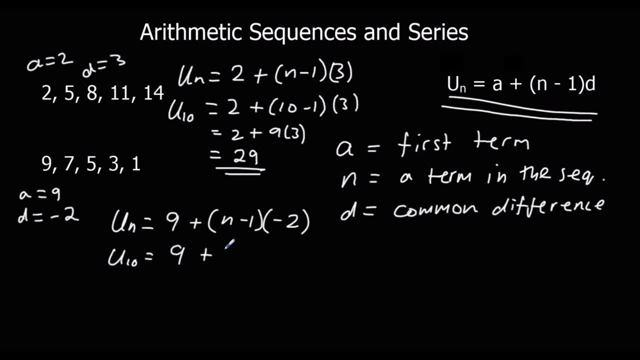 the tenth term, u10, is 9 plus 10 minus 1 times minus 2,, which is 9 plus 9, lots of minus 2,, which is 9 minus 18,, which is minus 9.. So the tenth term of this second sequence is minus 9.. 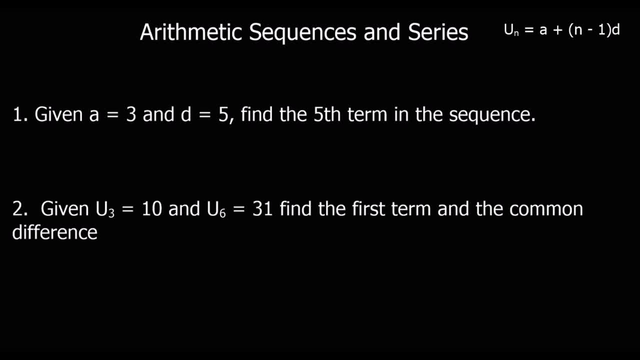 OK, so we're going to practice using the formula. So we've got the formula up here. un is a plus n minus 1 times the difference, So a, the first term is 3, and it goes up in fives. 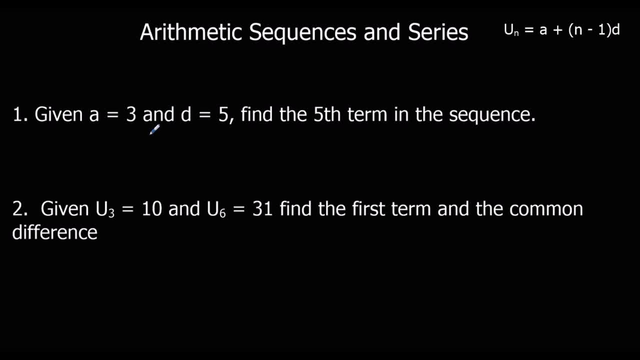 What is the fifth term? So u5,. the fifth term is a: 3, plus n minus 1.. So we want the fifth term, so n is 5,, 5 minus 1, lots of d, which is 5.. 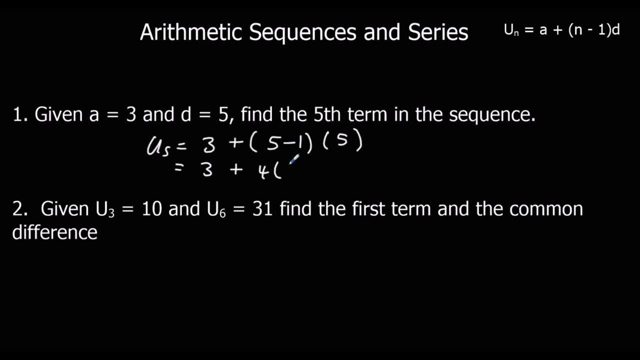 So it's 3 plus 4 fives. 4 fives are 20, plus 3, 23.. Secondly, we've been given two terms. We've got two terms in the sequence and we need to find the first term and the common difference. 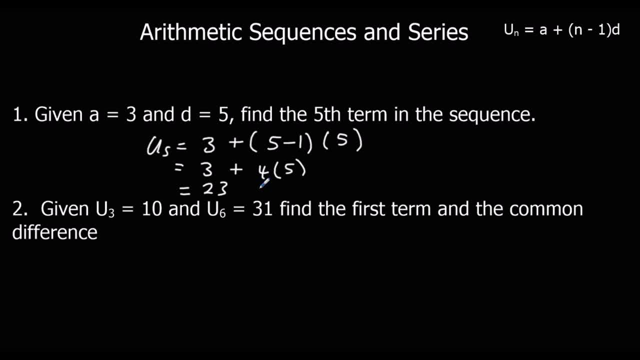 Secondly, we've been given two terms in the sequence. And we need to find the first term and the common difference. So this is simultaneous equations. We've got two equations. Well, when we make them, we've got two equations and two unknowns, the first term and the common difference. So u3 is 10. So we've got n is 3. So 10, u3 equals 10. So I'm going to change this to 10, equals a plus 3. So we've got 3 minus 1. Right, 3 minus 1 times d. So 10 equals a plus 2d. Secondly, 31 equals a plus 6 minus 1, because n is 6 for this one. 6 minus 1 times d. 31 is a plus 5d. And so we've got simultaneous equations. 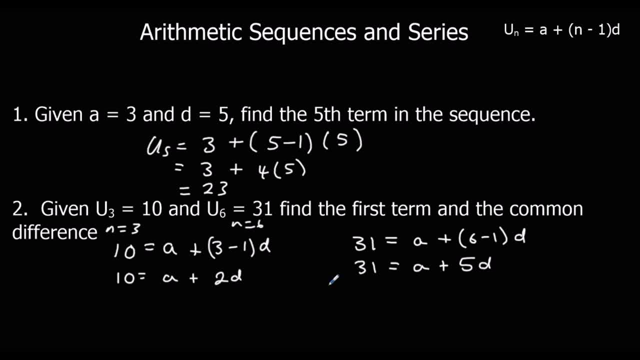 What we can do is we can write this first one here, underneath the second one, and take away. So we've got 21. The a's cancel, equals 3d. So d must be 7. And I can use that d is 7, and I'll substitute it in. a plus 2, 7. 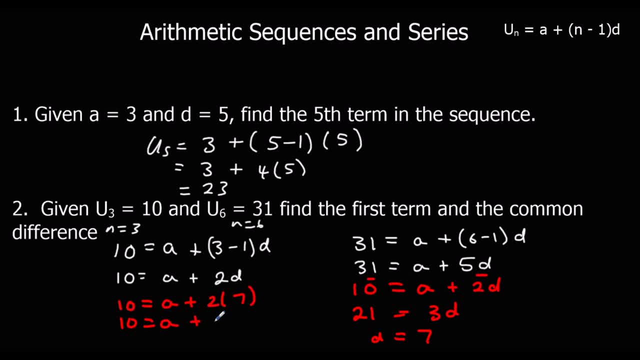 10 equals a plus 14 minus 14 from both sides so a must be minus 4 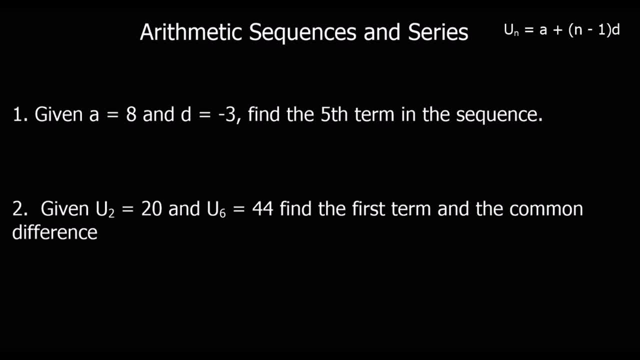 okay so the same sort of questions you can pause the video and give them a go 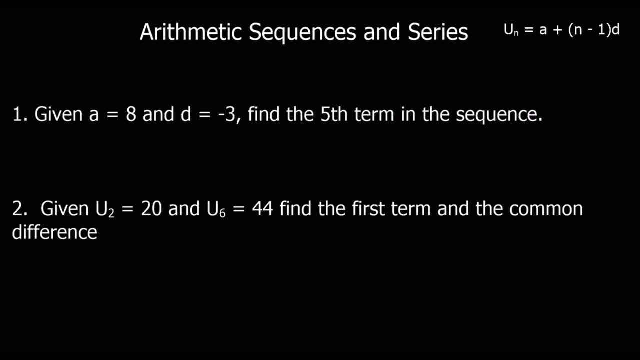 okay so a is 8 d is minus 3 we can find the fifth term so the fifth term is called u5 uh is a plus 5 minus 1 times d which is minus 3 so 8 plus 4 times minus 3 and 8 minus 12 8 minus 12 is minus 4 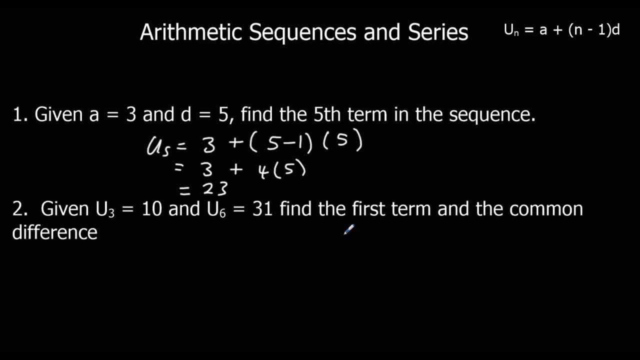 So this is simultaneous equations. We've got two equations. well, when we make them, we've got two equations and two unknowns: the first term and the common difference, So u3 is 10, so we've got n is 3,, so 10, u3 equals 10, so I'm going to change this to 10,. 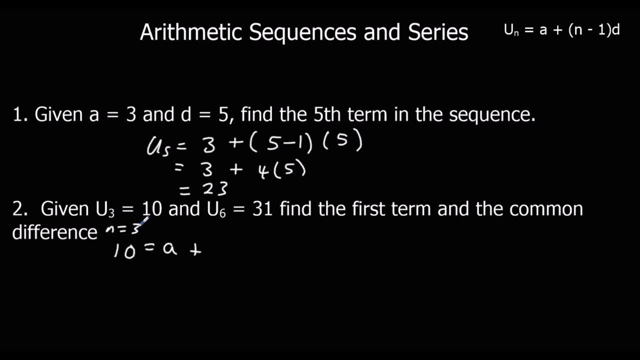 equals a Plus 3 minus 1,. all right, 3 minus 1 times d. so 10 equals a plus 2d. Secondly, 31 equals a plus 6 minus 1, because n is 6 for this one: 6 minus 1 times d, 31. 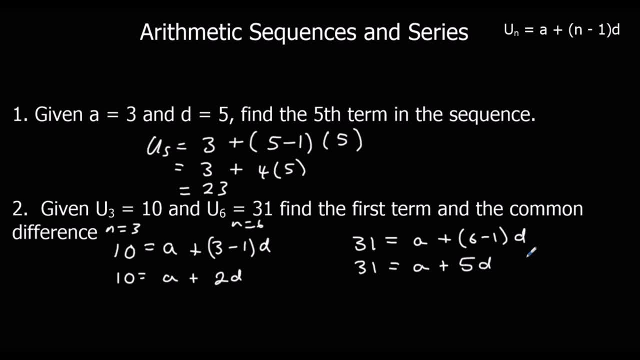 is a plus 5d, And so we've got a similar equation. We've got simultaneous equations. What we can do is we can write this first one here underneath the second one and take away, So we've got 21,. the a's cancel equals 3d, so d must be 7, and I can use that d is 7,. 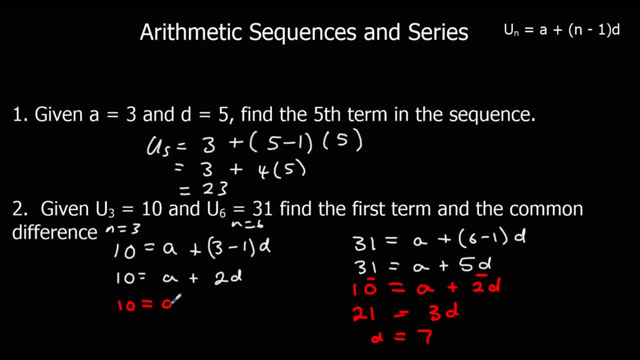 and I'll substitute it in: A equals 3d, So d must be 7.. A plus 2, 7s 10 equals a plus 14, minus 14 from both sides, so a must be minus 4.. 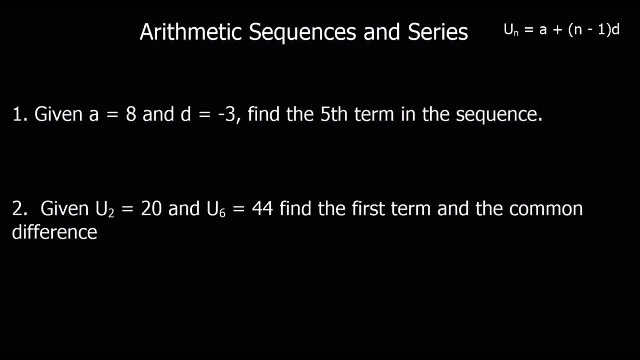